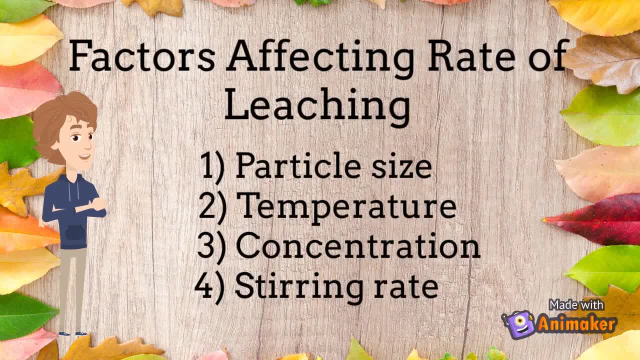 soy bean with the liquid solvent water. Factors affecting the rate of leaching includes particle size, temperature, concentration or reagent and stirring rate. To add on smaller particle size, higher temperature, higher concentration of reagent and higher stirring rate gives higher 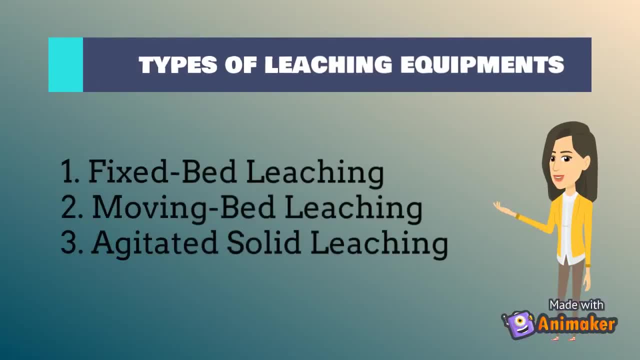 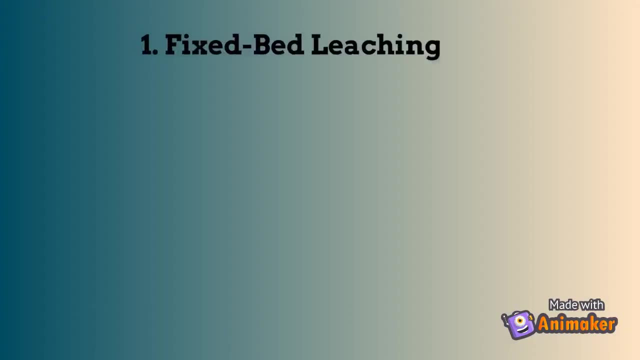 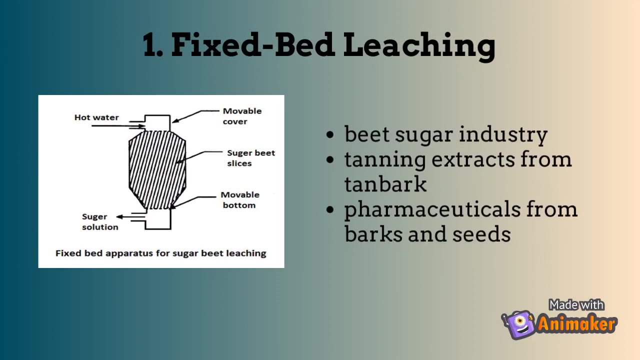 rate of leaching. There are three types of leaching equipments: Fixed bed leaching, Moving Bed leaching And agitated solid leaching. Fixed bed leaching is used in processes such as beet sugar extraction, extraction of tanning extracts from tan bark and extraction of pharmaceuticals from barks and seeds. 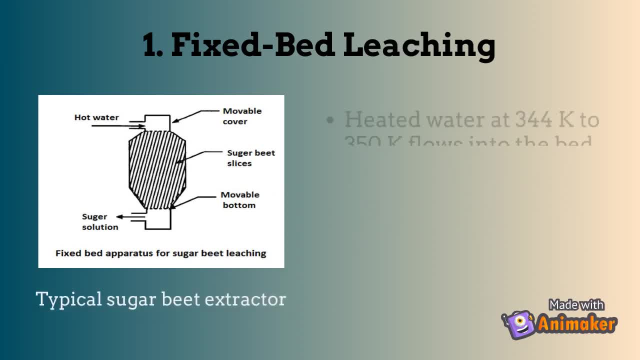 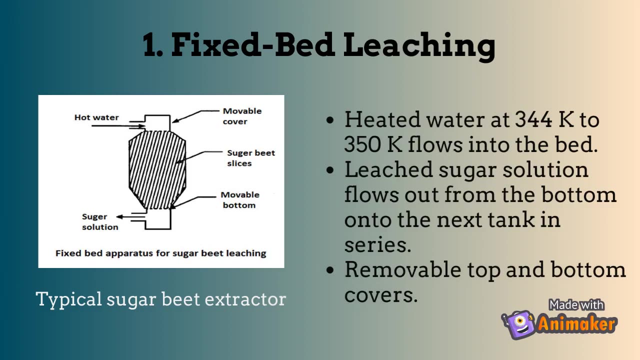 This figure shows a typical sugar beet extractor. Heated water at 344 Kelvin to 350 Kelvin flows into the bed to leach out the sugar. The leached sugar solution flows out the bottom onto the next tank in series. The top and bottom covers are removable so that the leached beets can be removed and a fresh charge. 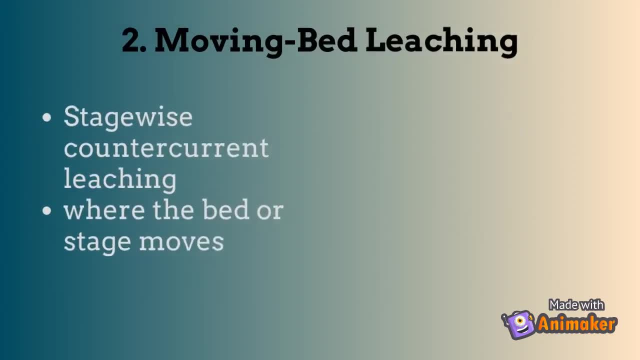 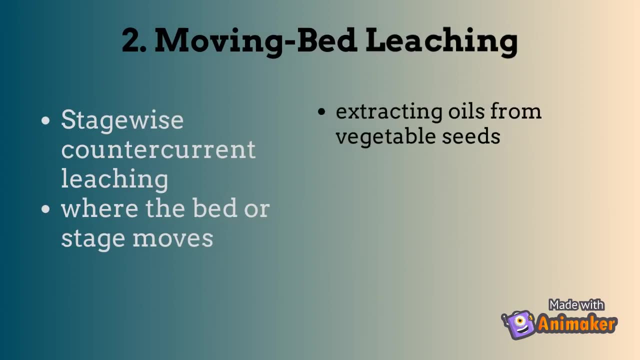 added For moving bed leaching. there are a number of devices for stage-wise countercurrent leaching where the bed moves instead of being stationary. These are widely used in extracting oil from vegetable seeds such as peanuts and soybeans. The solvents are usually petroleum products. 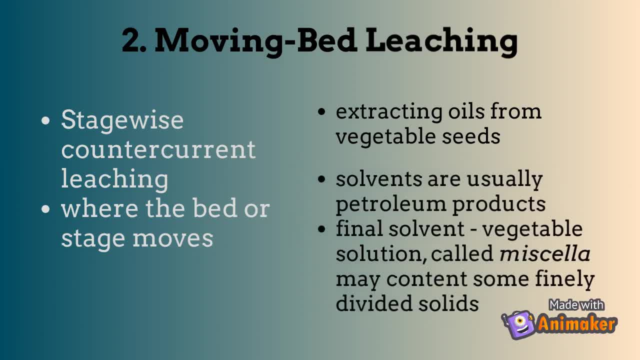 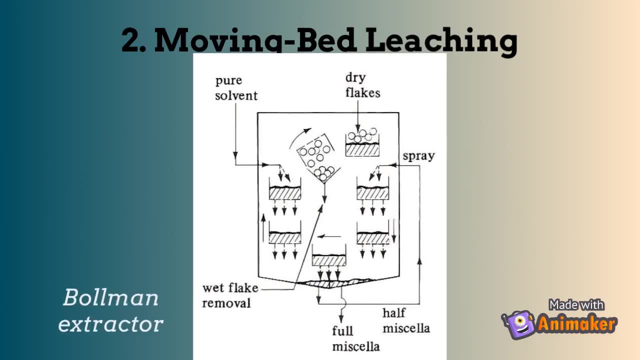 such as hexane. The final solvent, vegetable solution called misola, is a liquid that is leached from the bottom to the top. The liquid is leached from the bottom to the top and some finely divided solid. This figure shows the Bauman extractor, an enclosed moving bed. 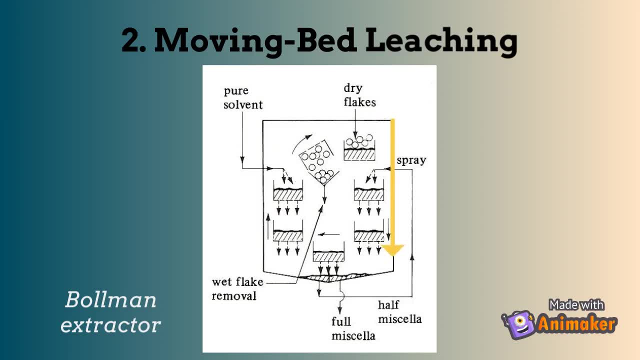 bucket elevator device. Dry flakes are added at the upper right to a perforated bucket. As the buckets on the right side descend, they are leached by a dilute solution of oil and solvent called half-misola. This liquid percolates downward through the moving buckets and is collected at the 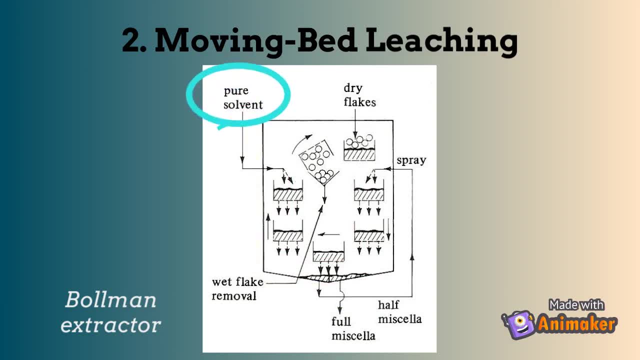 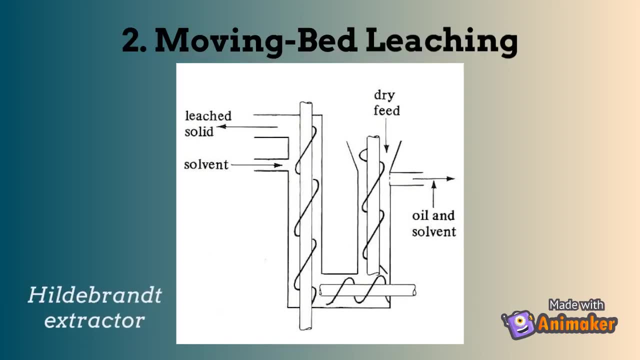 bottom as the strong solution or full misola. The liquid is then recharged countercurrently by fresh solvent sprayed on top bucket. The wet flakes are removed continuously. Figure shows Hildebrandt extractor. It consists of three screw conveyors arranged in U-shape. The solids are charged at the top right, convey downward across the bottom. 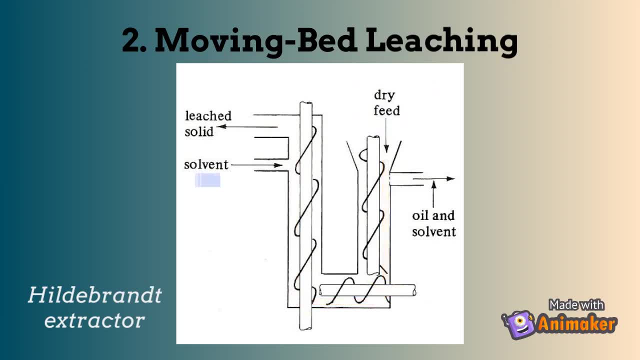 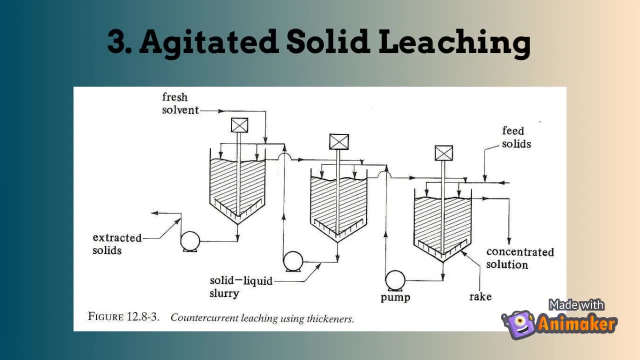 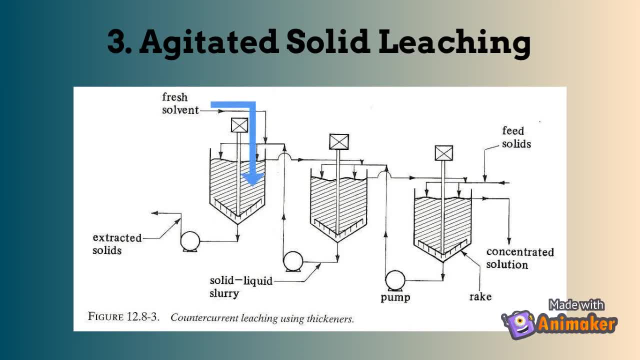 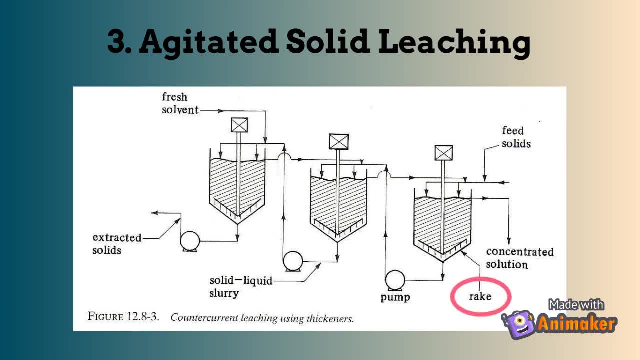 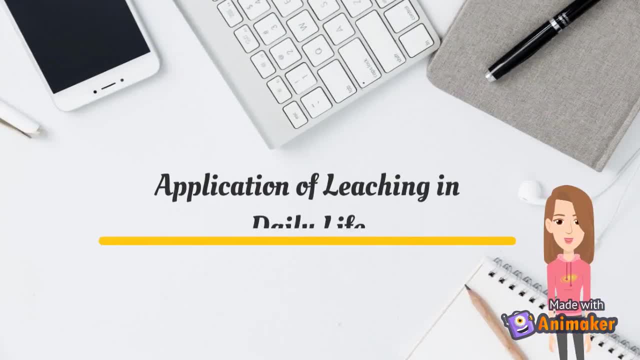 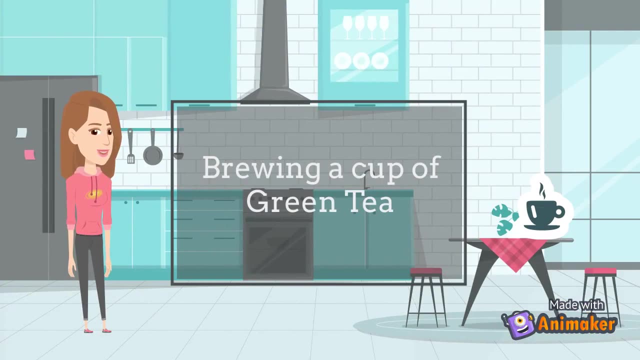 The slowly rotating rake moves the solids to the bottom discharge. The solids, together with some liquid, are pumped as a slurry to the next tank. Application of leaching in daily life. Leaching happens every day in our daily life. The most common leaching process that you might have witnessed before is the brewing of a cup of green tea. 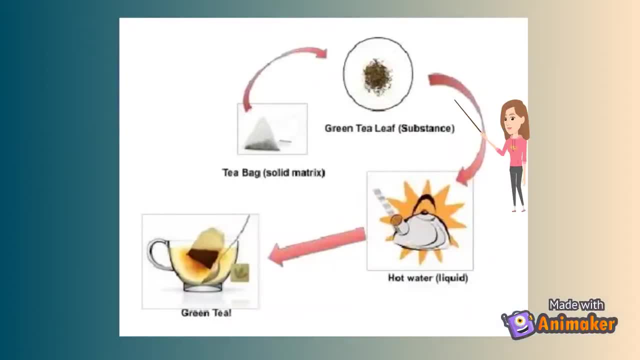 From here we can see that the teabag is our solid matrix. Green tea leaf flavor will be our desired substance to be extracted. Hot water is the liquid used to facilitates the ability to remove or extract the given substance from solid matrix. Finally, this results in a drinkable tea solvent. 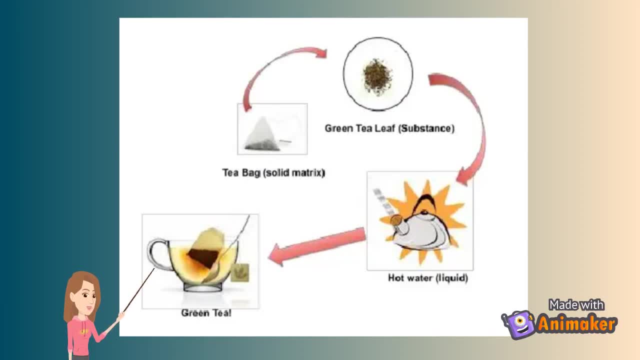 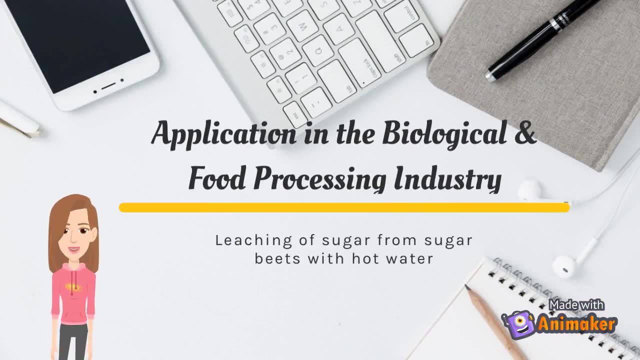 with dissolved flavors, with the completely depleted tea leaf residue solid carrier phase remaining in the teabag. Now we will discuss on the application of leaching in biological and food processing industry. The type of equipment used for leaching of sugar from sugar beets is: 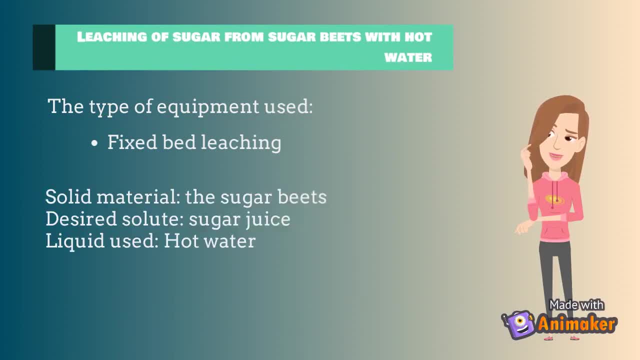 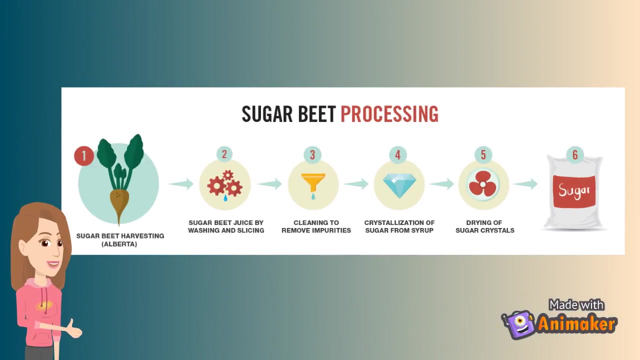 the fixed bed leaching In the leaching process. sugar beets are the solid materials. The desired solute that we want to extract is the sugar juice. Both of these are in contact with the liquid solvent, which is the hot water for leaching to occur. Sugar beet processing involving six 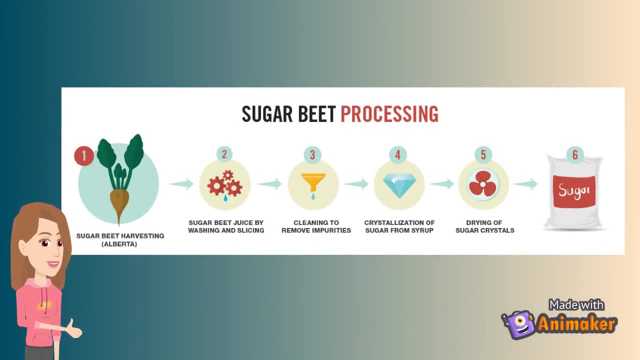 steps. First, the sugar beets are harvested from the farm. Second, the sugar beets are washed and sliced to extract the juice and separate it from the plant material. Third, the juice is cleaned to remove impurities and extra color to produce the sugar syrup. Then they are crystallized Finally. 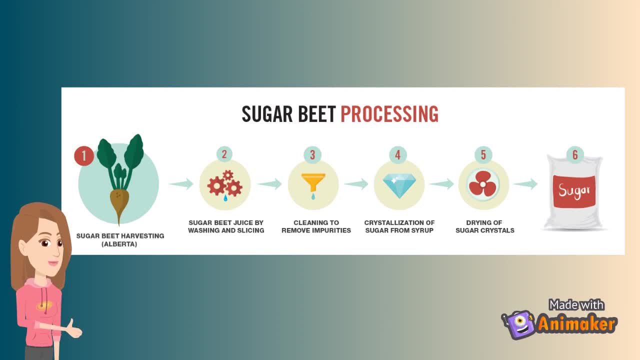 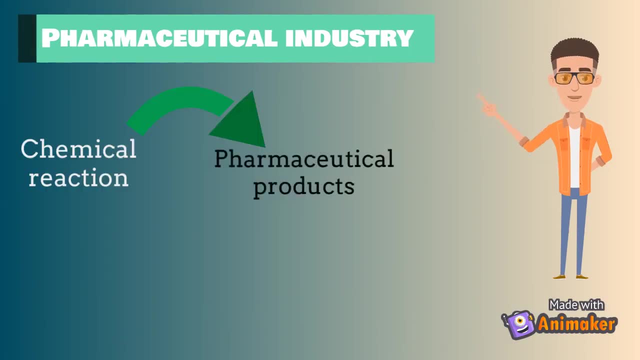 the crystallized sugar is dried and packed for distribution. Besides, the pharmaceutical industry is involved in leaching process. The products from pharmaceutical manufacturing processes are isolated using different separation processes, such as leaching, and the products are sent to the processing, to the formulation unit. Next, metal processing industry also. 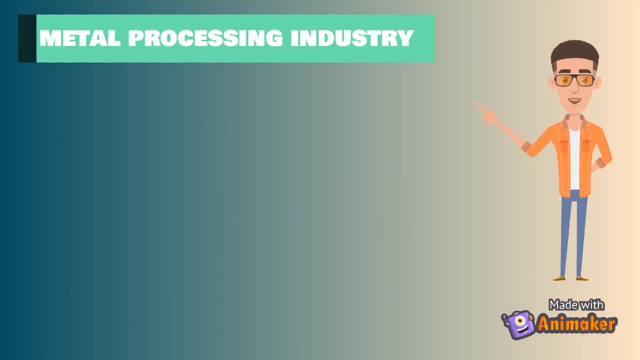 involved in leaching application. One of the examples is leaching of gold from its ore with aqueous cyanide solution. There are two types of gold leaching, which are heap leaching and vat leaching, or can be called as tank leaching. In vat leaching, the ore is mixed with cyanide. 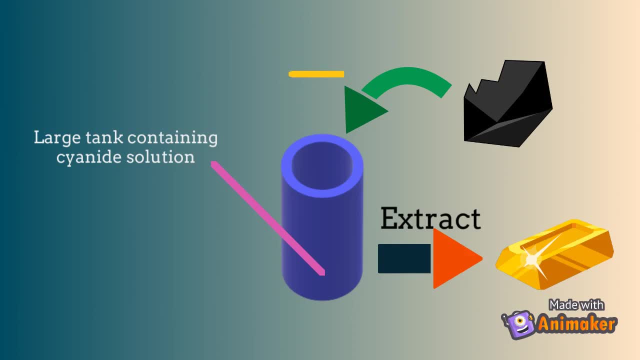 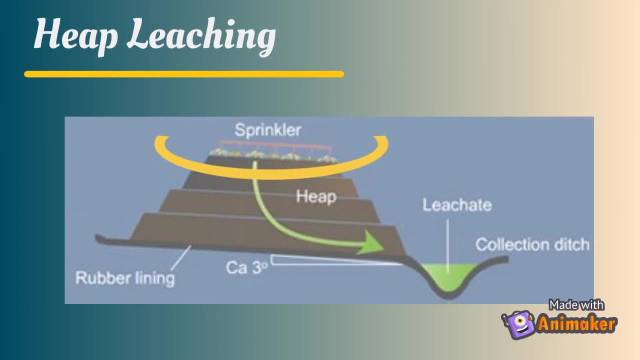 solution. The leaching process is called tank leaching. The leaching process is called tank leaching in large tanks to extract the gold In heap leaching cyanide solution is sprayed over huge heaps of crushed ore spread atop giant collection pads. As it trickles through the heap, the cyanide 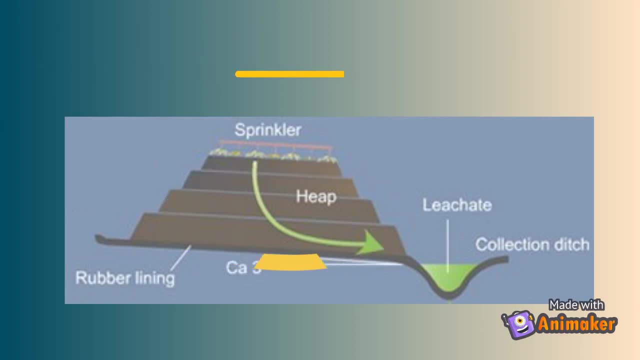 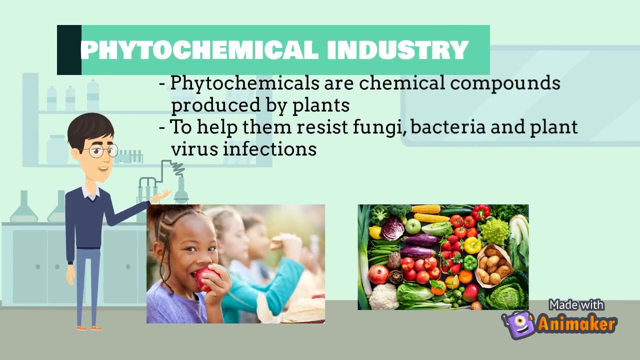 dissolves the gold from the ore into the solution. Lastly, the application of leaching process is phytochemical industry. Phytochemicals are chemical compounds produced by plants generally to help them resist fungi, bacteria and plant virus infections and also to prevent the production of bacteria and plant virus infections. 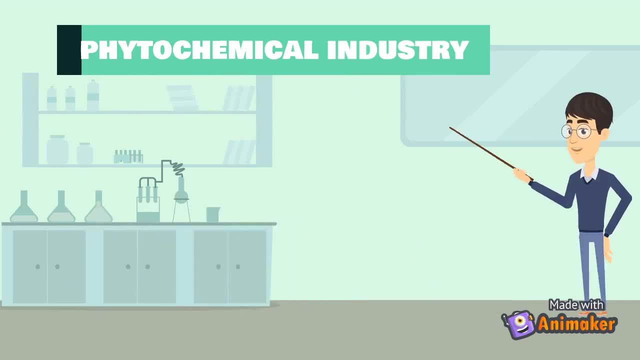 also consumption by insects and other animals. For instance, vitamins A, C, E and phenolic compounds found in plants all act as antioxidants. In order to obtain the photochemical from plants or herbs, leaching process is required. in this process, Multiple solvents have been commonly used to 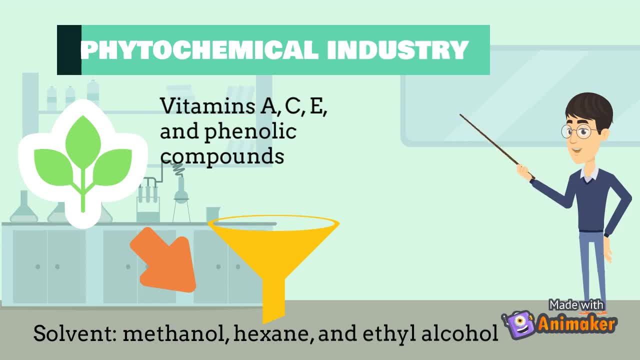 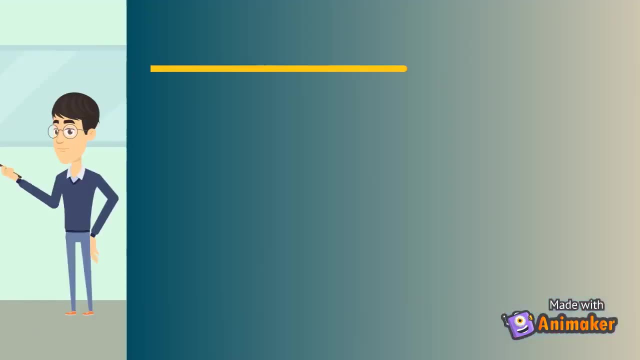 extract phytochemicals such as methanol, hexane and ethyl alcohol. In this process, the antioxidant liquid in the inlet plant is dissolved by using the hexane solvent. Then the enriched solvent will float a purification section to obtain a pure antioxidant liquid. 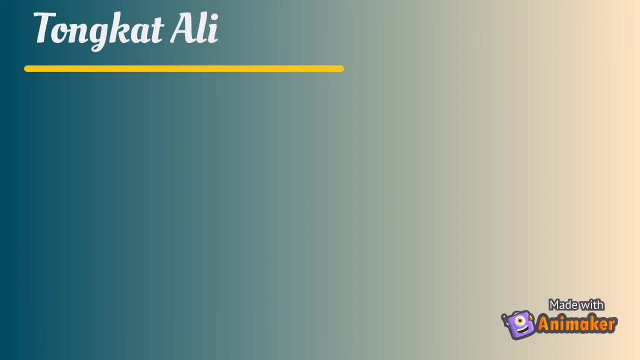 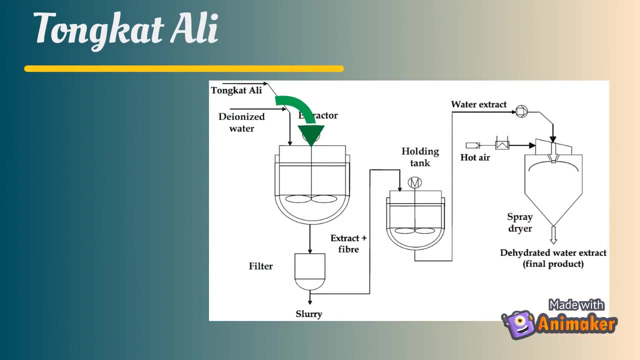 Tongkat Ali is one of the leaching applications in phytochemical industry. First Tongkat Ali root chips are sent to the extraction vessel to be extracted using the boiled water as a solvent. After the first stage of extraction, the extracted liquid is pumped and 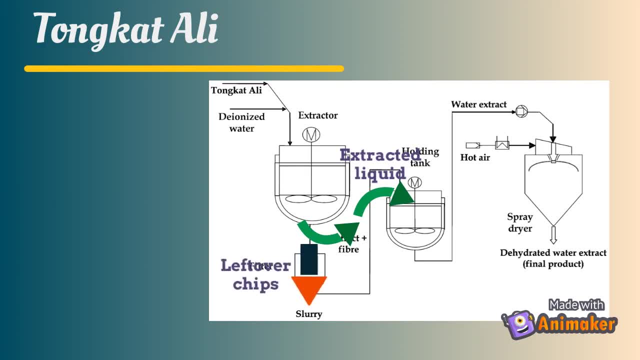 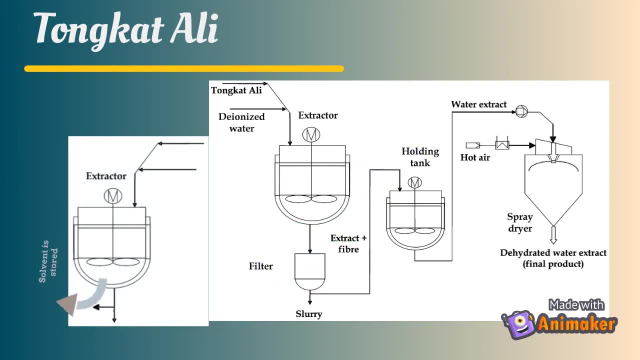 stored in a holding tank, while the leftover chips are then extracted again using fresh solvent in the second stage of extraction. After the second stage of extraction, the solvent is removed and stored for reuse in the following batch and the leftover chips are discharged. The extract from the first extraction stage is sent to the spray dryer to produce Tonka Ali extract powder.